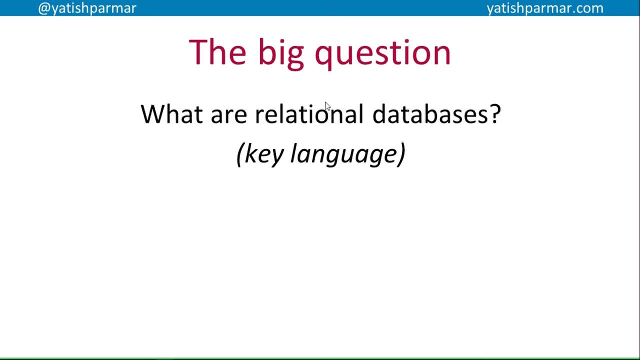 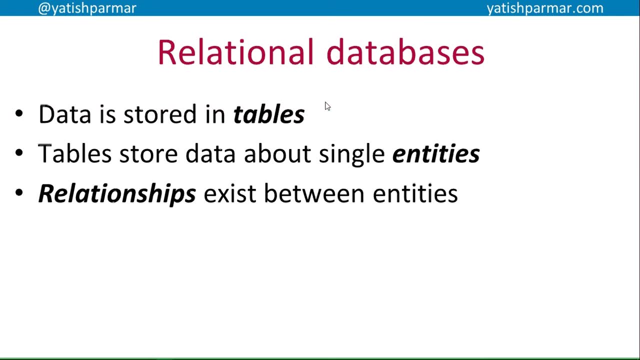 look at actually anti-relational diagrams in much detail. That's in the next one. This one is focusing on the key language that you need to understand. So with a relational database, basically what we're saying is it's opposite to flat file. So you had a single table storing all. 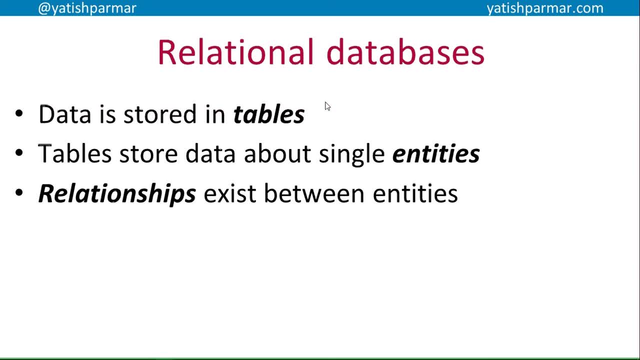 the data. Here we're splitting up the data. It's stored across different tables. The tables are storing data about single entities and relationships exist between the entities. An entity, basically, is a real world thing that can be modeled through the data that represents it. 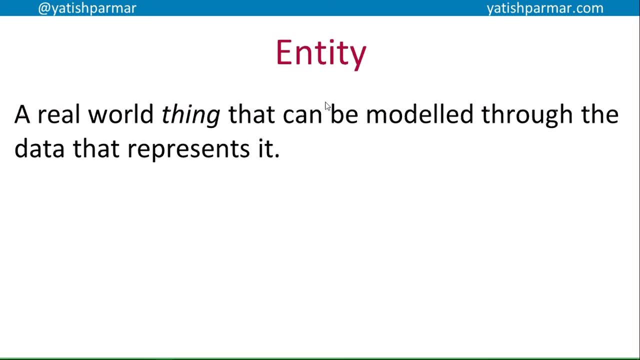 This is the only time you'll hear me use the word thing to describe something. Okay, it's a very woolly concept That's difficult to explain. So these are examples of entities. For example, car would be an entity and be modeled through the data, For example the VIN, vehicle identity number identification. 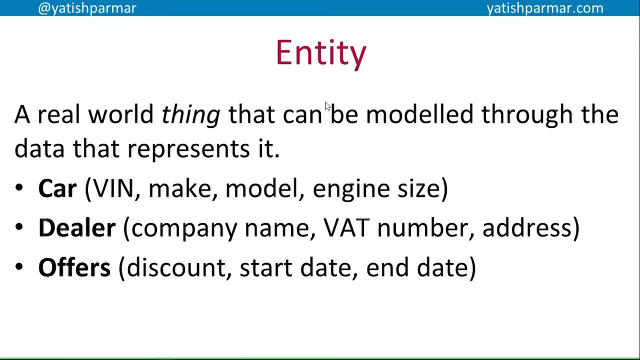 number, the mate, model, engine size, et cetera, et cetera. Dealer would be the company name, the VAT number, the address, the telephone number then offers. So you can see car and dealer are concrete, tangible things that we see, You can touch, feel whatever. it is Okay, Sometimes an. 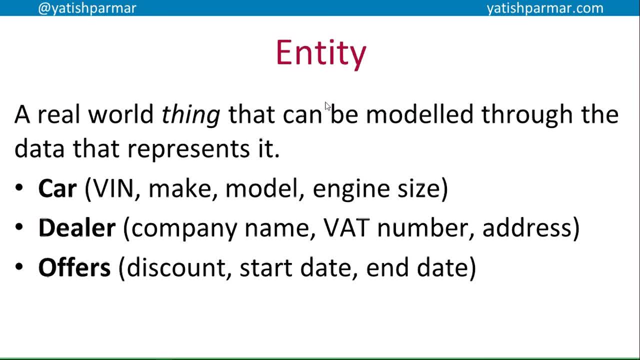 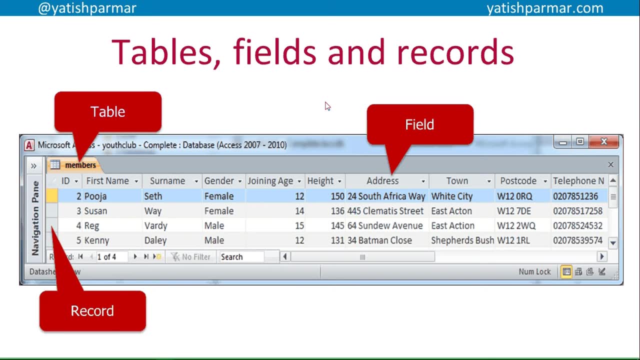 entity might be something that's abstract, But still something that exists and it can be modeled through the data represents it, because an offer can be represented by the discount, the start date, the end date, the products that it applies to, et cetera. Okay, So this was a familiar screenshot, maybe for you looking at. 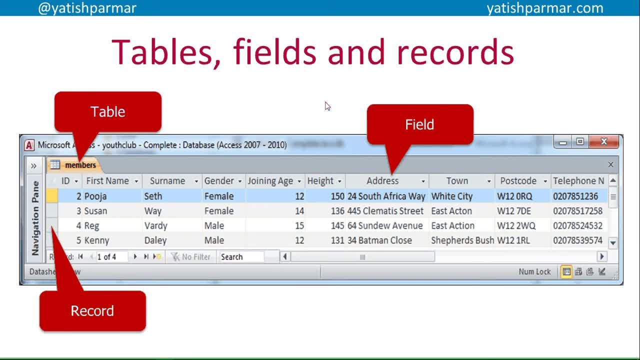 Microsoft Access here. This was from a couple of videos back. It talks about tables, fields and records. Okay, So table is the collection of data, A record is the data about one particular person, for example, And then a field is the individual bits of data that make up the table. 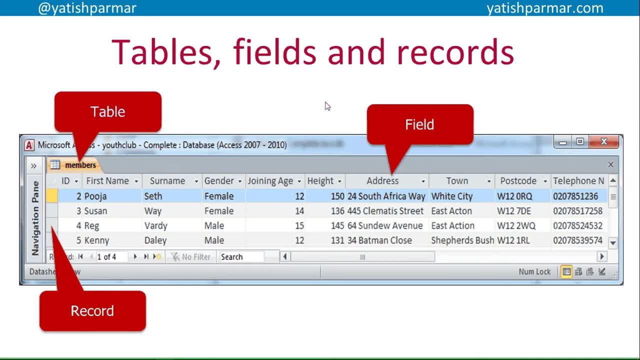 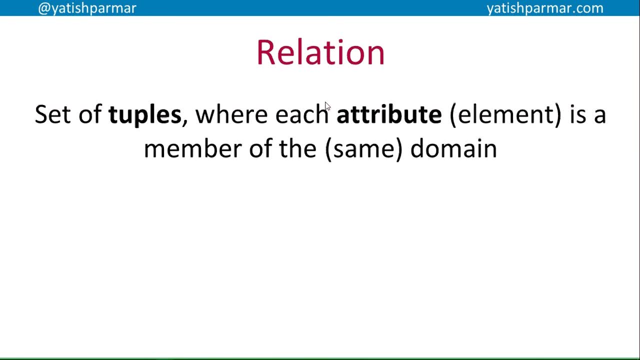 Okay, Or make up a record. Some people would define a field as the column heading- Okay. Well, another name for a table is a relation: Okay, And it can be defined as a set of tuples where each attribute or an element is a member of the same domain. Okay, We say D little j is a member. 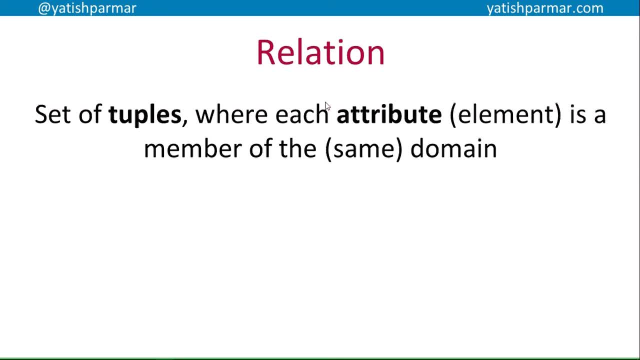 of the domain D big J. All right, That's, I think, voice or chord. I forget who it is. is definition All right? So the next question you're going to ask me is: what is a tuple? All right So. 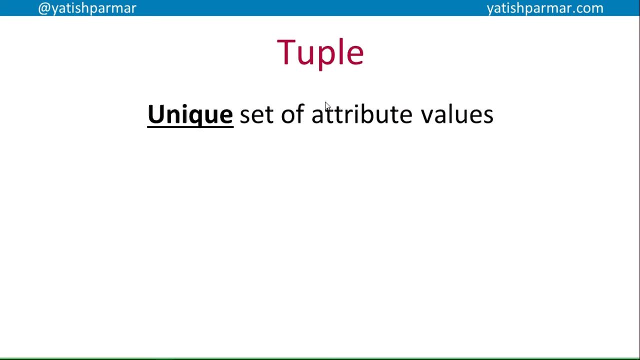 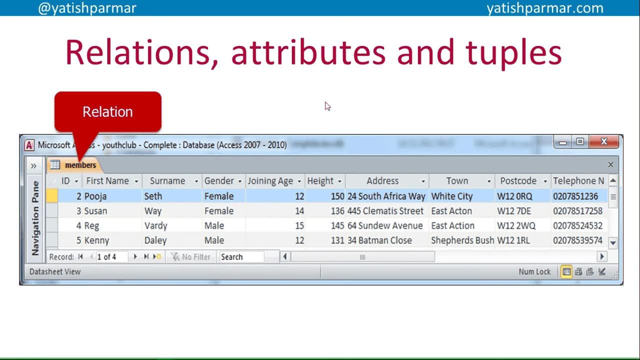 a tuple is a unique set of attribute values. You're like: huh, What does that mean? Well, if we look at the same screenshot again. but we can say a relation is the table. Okay, The attributes are the items of data that make up the table And therefore, 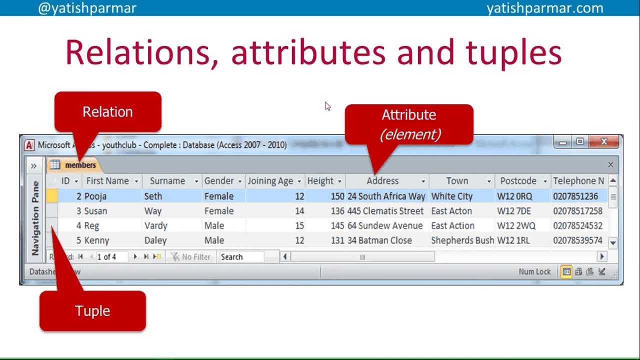 a tuple being a unique combination of attributes. So a tuple is a row within the table, All right. So a tuple is a row in a relational database, a row in a table in a relational database, Okay. So same screenshot, slightly different names. Okay, You should be able to relate relation attribute. 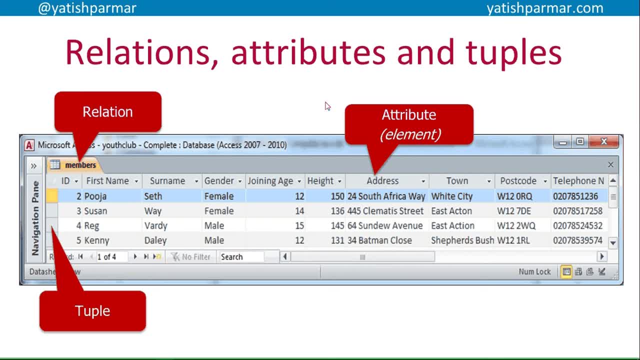 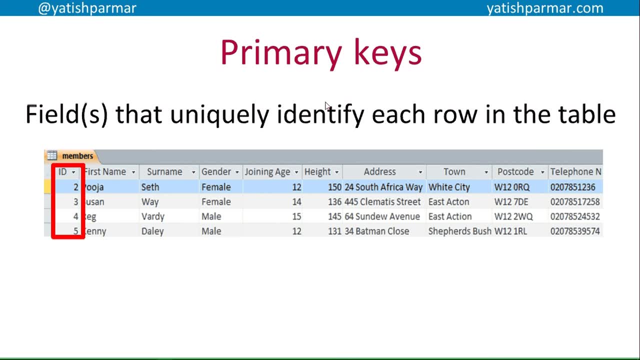 table, a tuple to table fields and records. So primary keys, if you remember, are the fields that uniquely identify each row in the table. So here we have a key data ID field and that is used to uniquely identify each member of this. I think this was like a youth club. 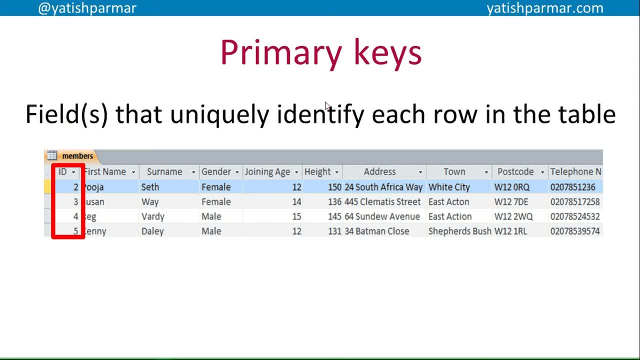 database that I made for a lesson some couple of years back. All right, For those of you who are really being nerdy about this, the ID field is actually what we call a surrogate key, because it's an artificial key that we've created to represent each person. A natural key would be: 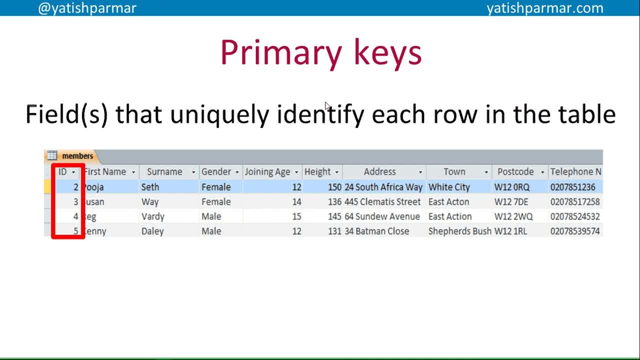 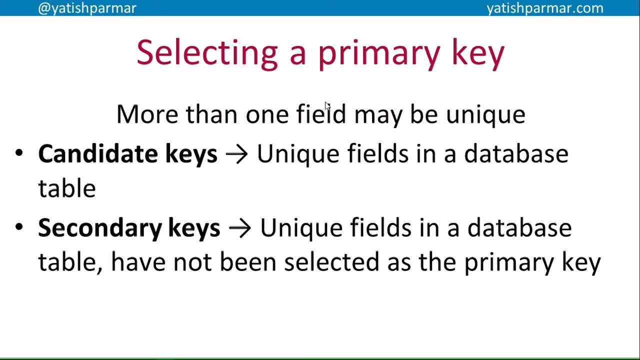 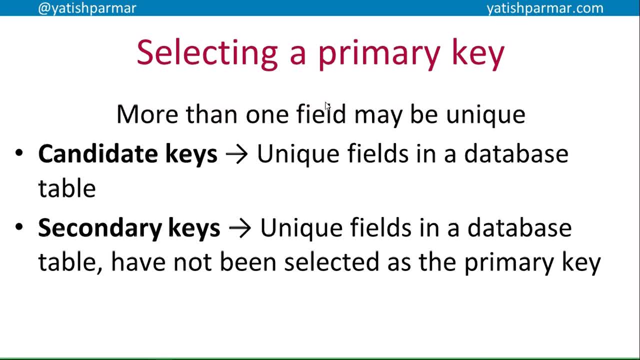 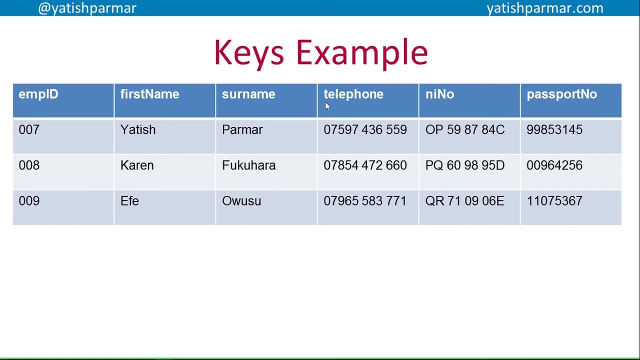 which are all of the unique fields in a relation, And the secondary keys are the unique fields in a database table which have not been selected as a primary key. Okay, So, for example, this could be a database table where we're storing data about the employees. So we've 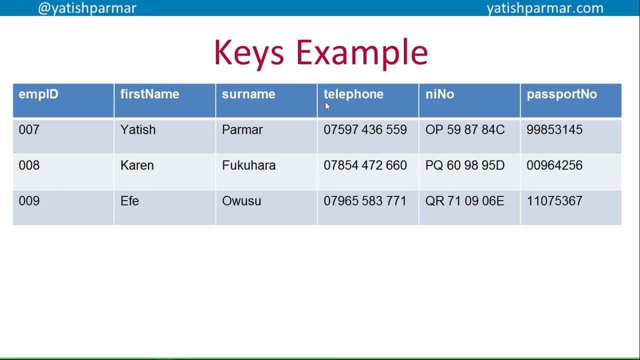 got the employee ID: first name, surname, telephone number, national insurance number, passport number. Out of that there are actually three other fields. Sorry, there are a number of fields that are unique because the employee ID, the telephone number, the national insurance number. 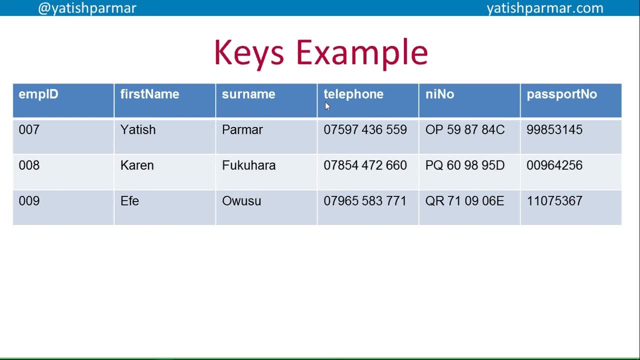 the passport number. they're all unique. Everyone has different telephone numbers, national insurance, passport numbers. Okay, So the candidate keys could be those four fields of which we choose one as the primary key. So the employee ID we've made the primary key. 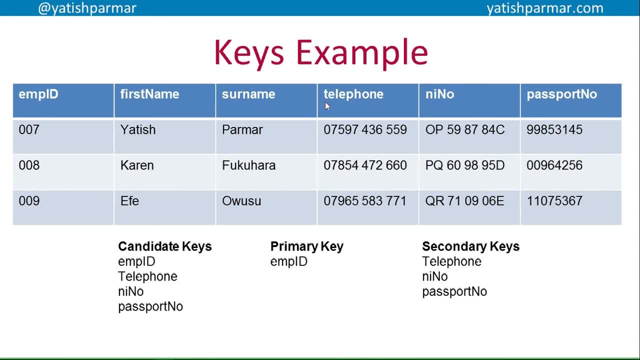 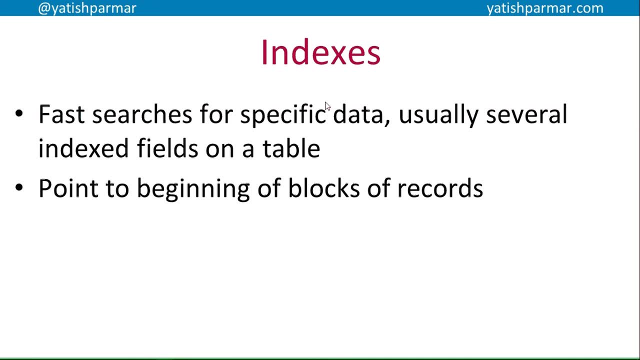 So the secondary keys would be the telephone number, national insurance number and the passport number. Now, following on from that, okay, you may remember that we talked about index, For example. we have index sequential records. So we've got, you know, those fast searches for. 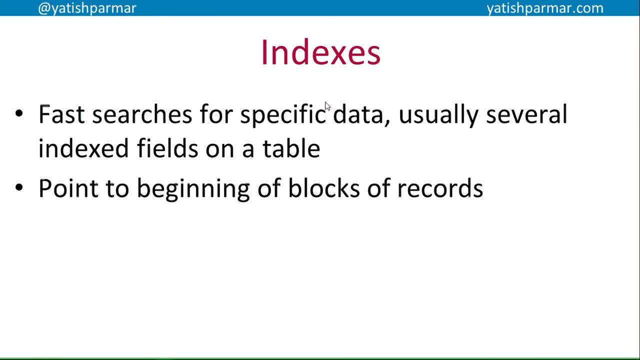 specific data. You know you've got millions of records in a database table. You want to find something quite quickly. You don't want to start at the beginning of the file and search all the way down. You want to jump to a certain block in that file and then start searching through those. 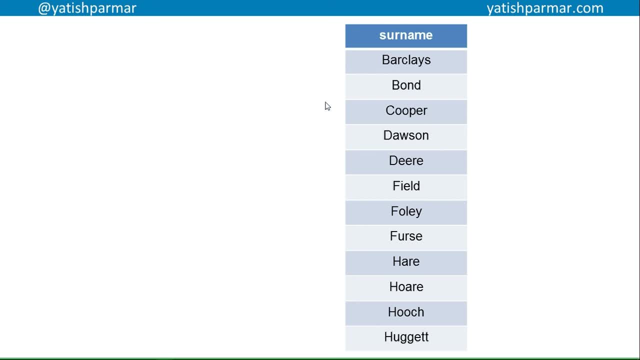 blocks. However, oh, let's do a quick demo of that just so you can visualize it. So if that is my database, a part of a table where I've got the surname field, you can see the index might look something like this, because then if I want to search for somebody whose surname begins with B, 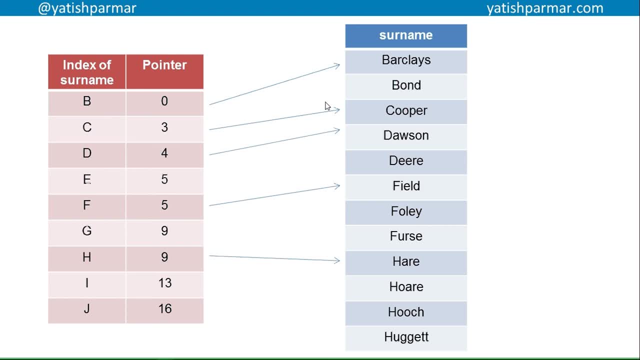 then I would look in the index, I'd jump to that position in the file and I'd be able to search each individual record there. Same thing: if I'm looking for someone whose surname started with F, I'd quickly jump down my index, find F, jump into the table and then start searching from there. 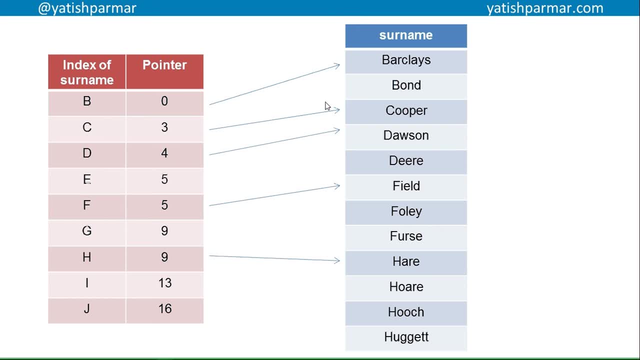 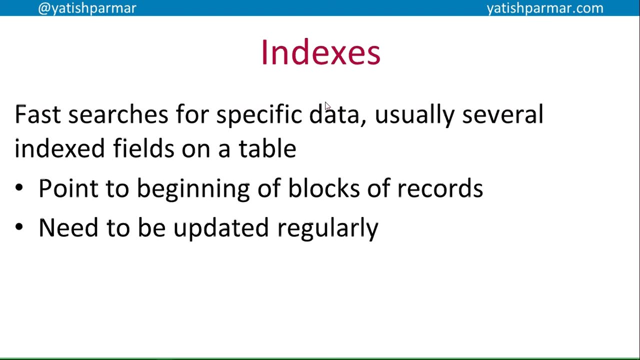 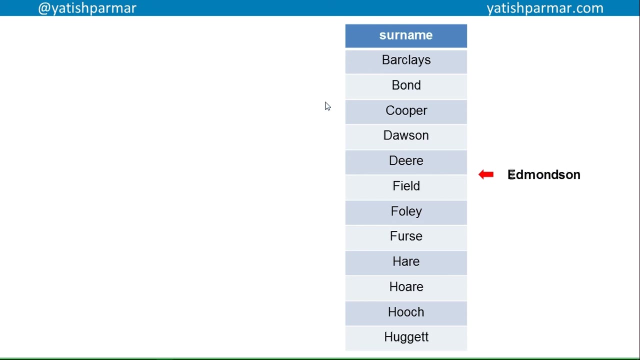 Okay, so it should speed up the process with which you search. Okay, just to think about with indexes, though they do need to be updated regularly. okay, because they point to the beginning of a block of records. So, for example, my original table where I want to insert the name Edmondson into there. 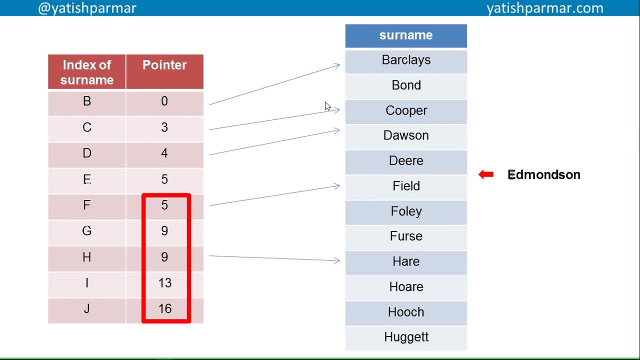 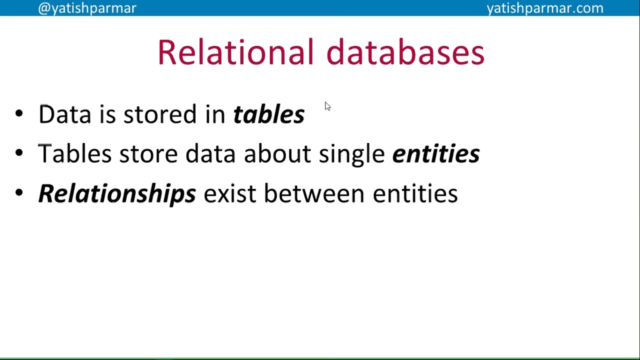 well, basically I'd have to update my index if I insert that Record, because if I don't update the index then it's going to be inaccurate for a number of records. It's actually not going to speed up the search. Okay, now with relational databases. 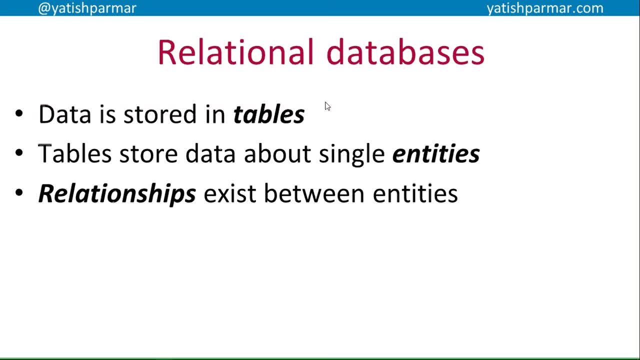 just going to show that my three bullet point definition from earlier. So data stored in tables: table storing data about single entities and the relationships that exist in between those entities. All right, so here's an example: relational database. Okay, there are. 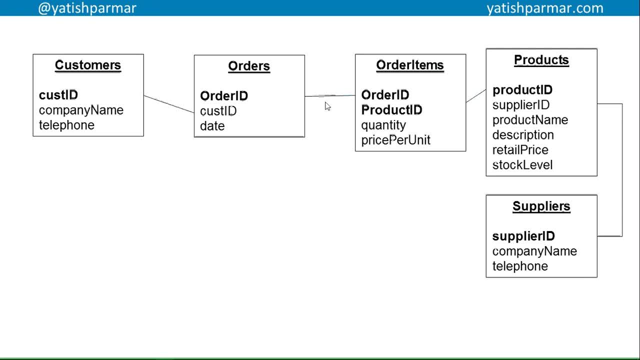 five tables: customers, orders, order items, products, suppliers- Okay, each of those tables has a primary key, All right. Now, in other tables there's also a foreign key. Okay, and the foreign key in, for example, the orders table is the customer ID, because it will link. 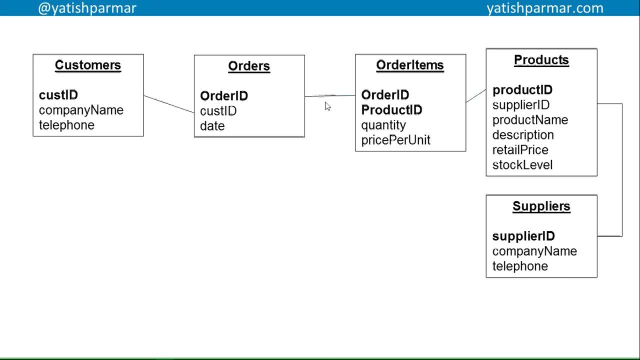 an order to a customer, So I don't need to have the company name and the company telephone number stored in the orders table. Okay, so I'm now removing all that duplicate Data, So you can see this immediately overcomes a problem that I showed with flat files in the 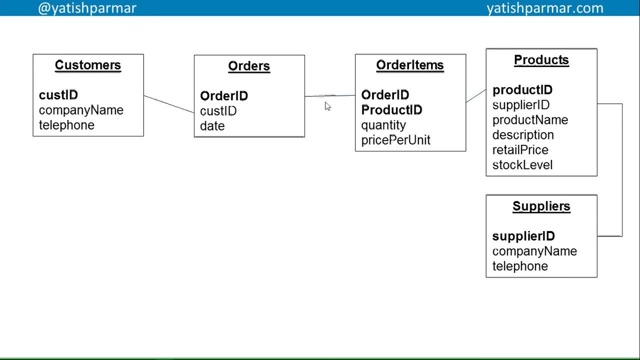 previous video, where you know you've got the same data in multiple tables, So where do you change it? In this case, all I ever need to do is, if the company changes the telephone number, change it in the customers table and any order that I search up, I will be able to find the most. 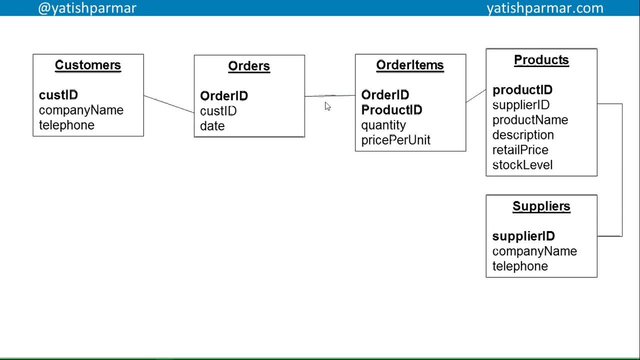 up to date relevant telephone number for that order. Okay, So you can remember. the primary key was a field that uniquely identified each row in the table Or each tuple. So you can see from that diagram the primary keys in bold. However, sometimes you 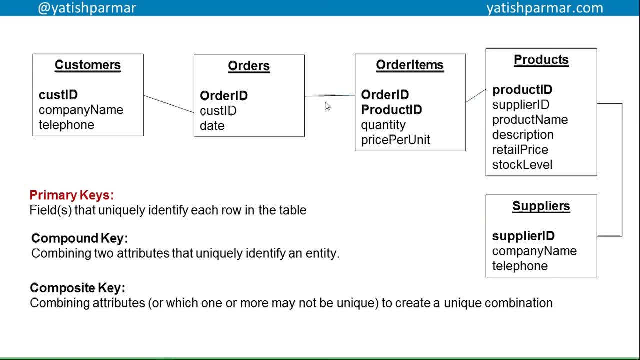 have what we call compound keys and composite keys. So compound keys, where you combine two attributes that uniquely identify an entity. So the order items table. you can see that we have orders and then we have products And every order will be made up of ordered items. So, in order to 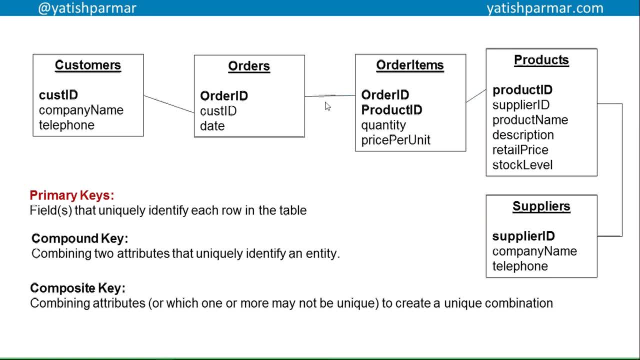 uniquely identify each order item. I've got a separate table where I can have a compound, a compound key. I've got an entity of the order ID and the product ID. okay, Those two, two things together would make a unique row in that table. So order five might have product six. Order five might also have product 17.. 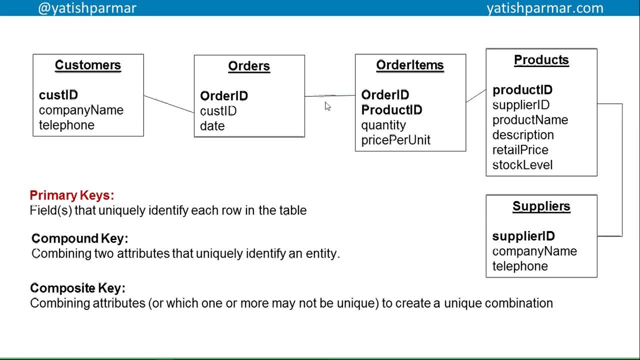 Those two things together make unique rows in that table. Okay, that's compound key. Composite key is where you combine attributes again, So you've got two or more fields together in combination, But one of those fields might not be unique. okay, But however, when 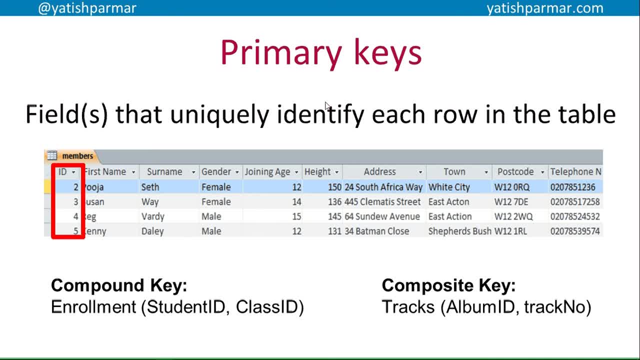 still combine them. you create a unique combination. so an example of that would be- you can see there in the bottom right hand side- if i had a music database where i have my cds, records all catalogued in it, each album album might be have a unique id, but the tracks are not unique because every